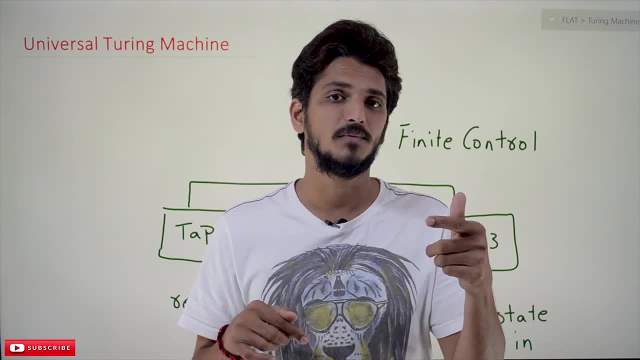 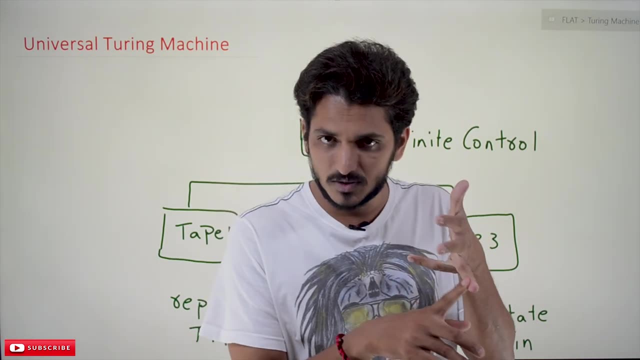 your computer is selecting the program and executing the program, But is it possible using Turing machine? No, we had a separate Turing machine. for addition, We had a separate Turing machine for subtraction. We had a separate Turing machine comparison. We are having it separately. 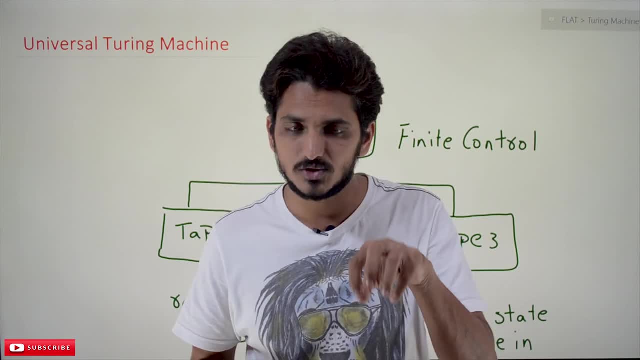 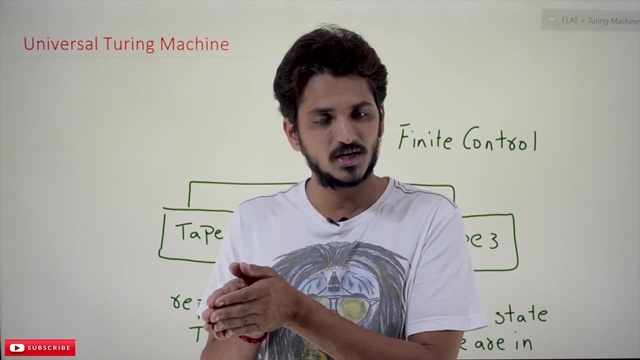 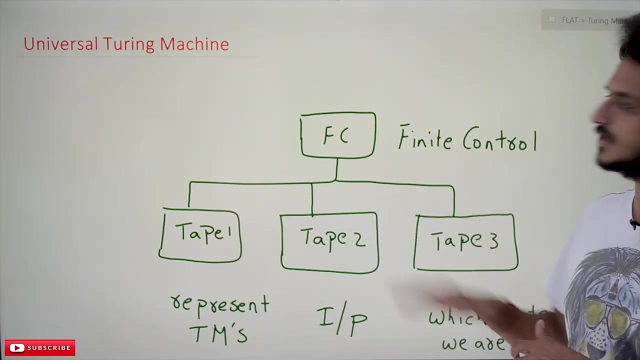 It is possible using universal Turing machine. Universal Turing machine is exactly works as our today's computers. What's universal Turing machine? How it is mentioned? Let's try to understand in this class. Yes, universal Turing machine consists of a finite control, finite control, FC. This is 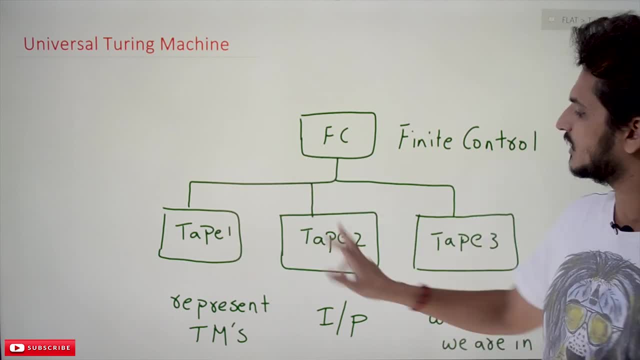 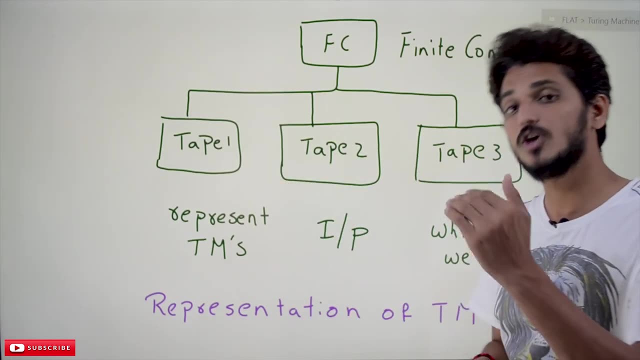 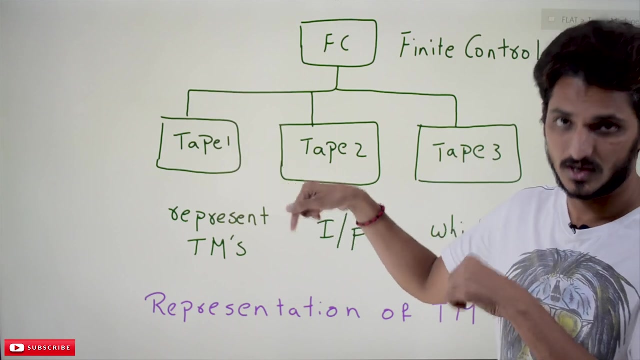 going to control and on this we are having three tapes: tape 1, tape 2 and tape 3.. Tape 1 is used to representation of the Turing machines. Suppose, if you are having a Turing machine for a addition, Yes, place it on it. How we place it, that we will try to understand at the end of the 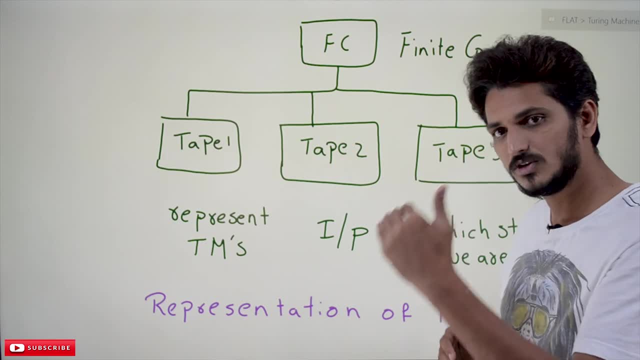 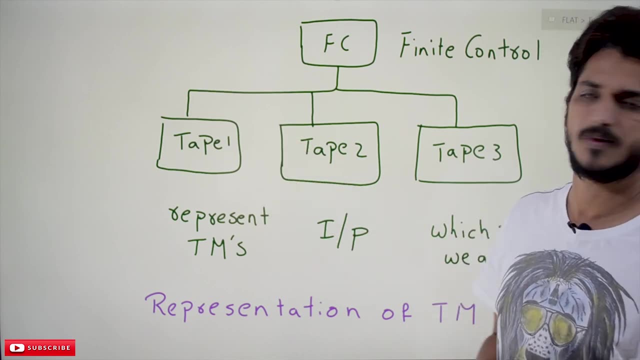 class. We will place on tape 1.. If you are having a Turing machine for subtraction, Yes, place it on tape 1.. This is how tape 1 is used to represent the Turing machines. Next one is tape 2, the input. 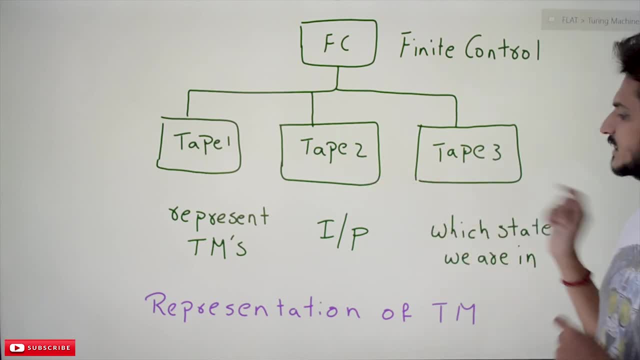 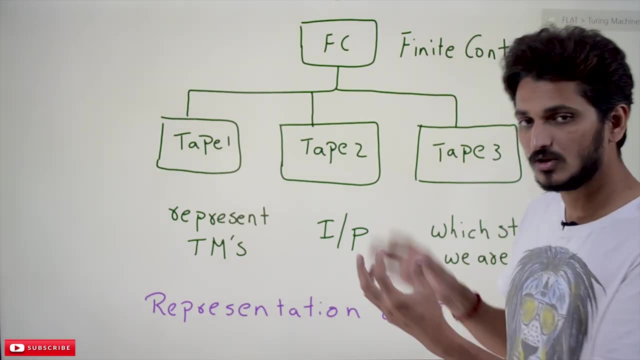 The input is provided and placed it on tape 2.. And next third tape is used to say that which state we are in. If you are executing a Turing machine, we are in Q2 state. Yes, in order to mention that we are using this third tape By using this finite control. 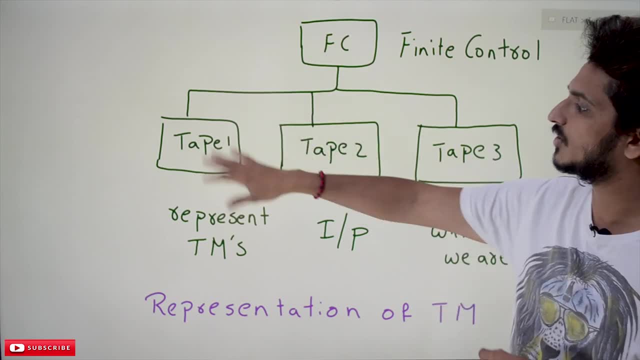 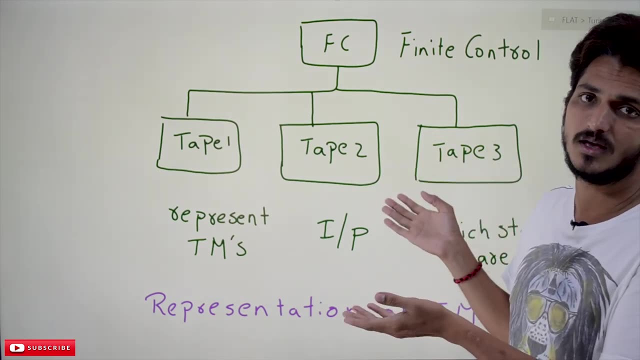 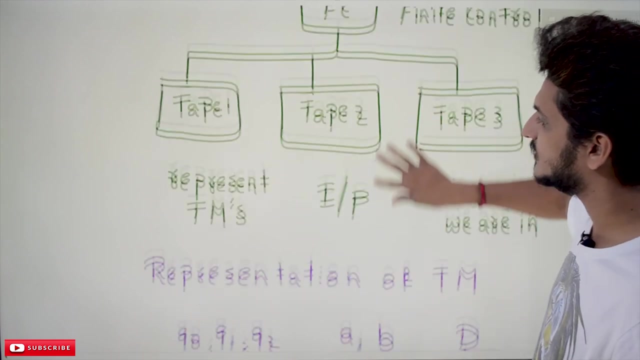 we can execute any Turing machine that are present on our tape 1 using the input by maintaining the states. This works exactly as our computer. The question is how we represent the Turing machines on tape 1.. That is the point we have to understand. Let's try to understand how we 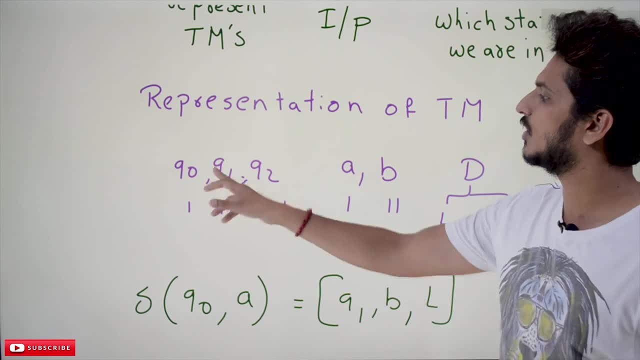 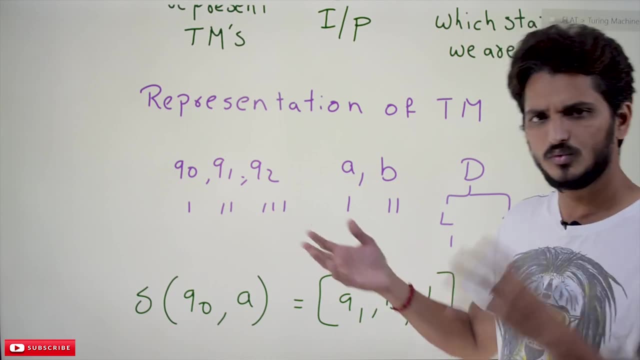 representation of Turing machine. Let's take example: Q0,, Q1, Q2 are the states that are present In our Turing machine. we are doing it as a coding system. How to do coding. This is the code which we have chosen in one of the text books. Is it compulsory to choose the same coding? No. 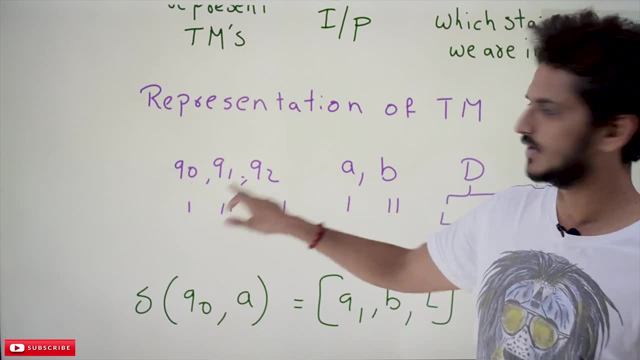 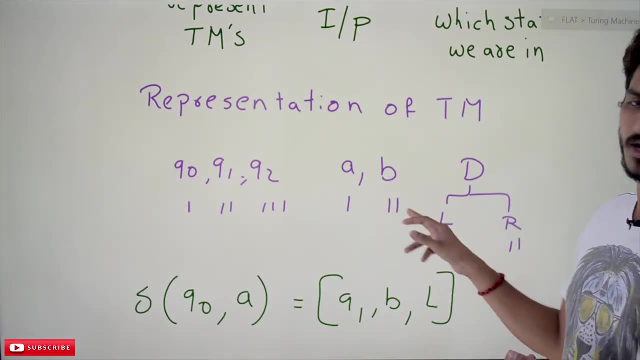 it's up to you, It's your wish. Q0 is given as single, 1. Q1 is given two: 1. Q2 given as three: 1. Our input symbols are tape symbols are 1. 1. 1. A, B are the symbols We have.